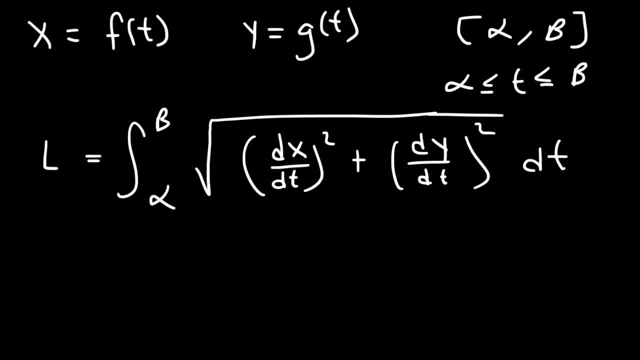 squared. So let's work on an example problem. So let's say that x is equal to 2 plus 16 t squared and y is equal to 5 plus 4 t cubed. And let's say t is restricted between 0 and. 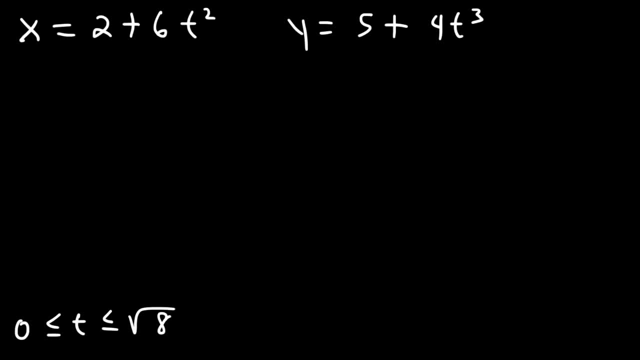 the square root of 8.. So go ahead and find the arc length from 0 to the square root of 8.. Feel free to pause the video Now. the first thing we need to do is calculate or determine a function for dx, dt and dy, dt. So dx over dt is going to be 6 times 2t, which is 12t. 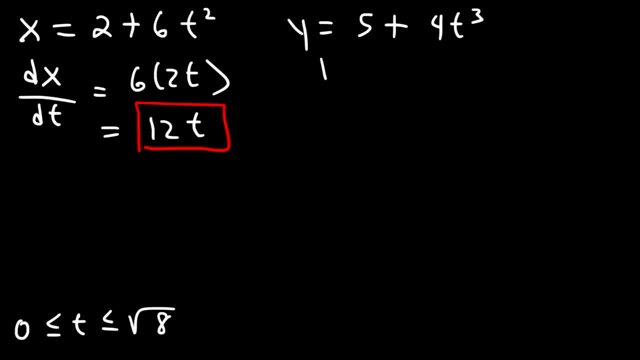 Now let's do the same for dy dt. The derivative of 5 is 0, and the derivative of t to the third power is 3t squared. So dy dt is going to be 12t squared. So now we can determine. 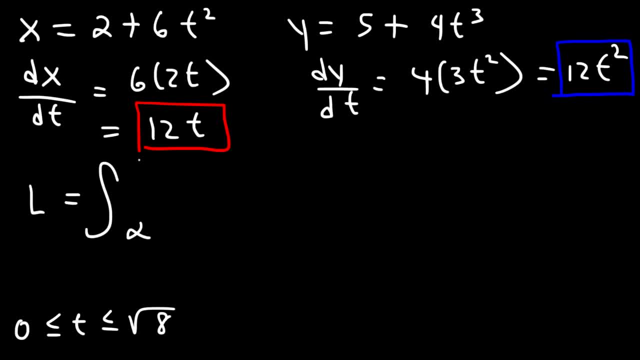 the arc length using this formula. So it's the integral from alpha to beta of the square root of dx, dt squared squared, which is 12t, plus dy over dt squared, which is 12t squared squared. Now, alpha is 0 and beta is the square root of 8.. 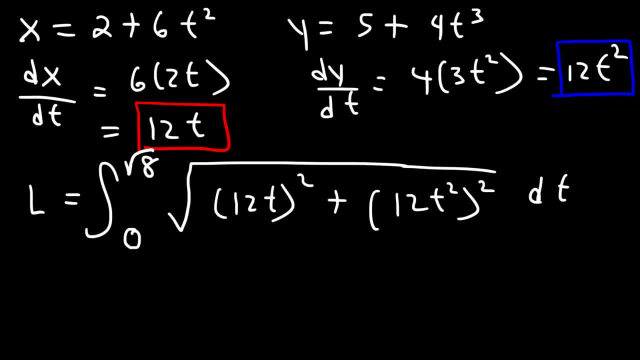 So what can we do to evaluate this integral? Let's begin by simplifying it: 12 squared is 144, so we're going to have 144t squared and 12t squared squared. that's going to be 144 and t squared squared is t. to the fourth power. 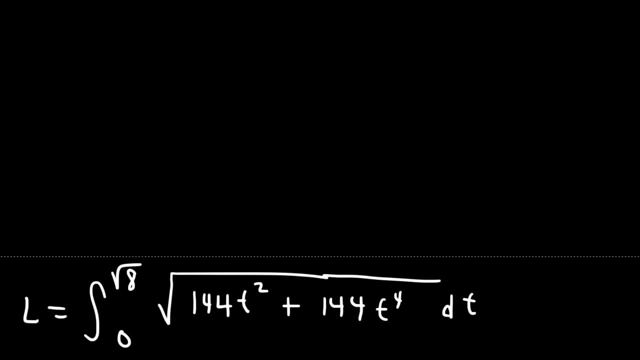 So what do you think we need to do at this point? We need to factor out the greatest common factor inside the square root, and so that's going to be 144t squared. If we take that out, we're going to be left with 1 plus t squared. 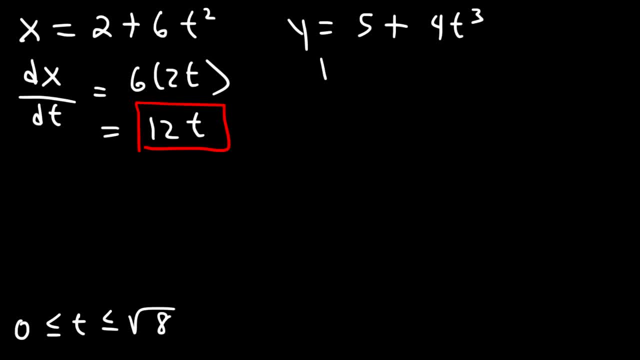 Now let's do the same for dy dt. The derivative of 5 is 0 and the derivative of t to the third power is 3t squared, So dy dt is going to be 12t squared. So now we can determine the. 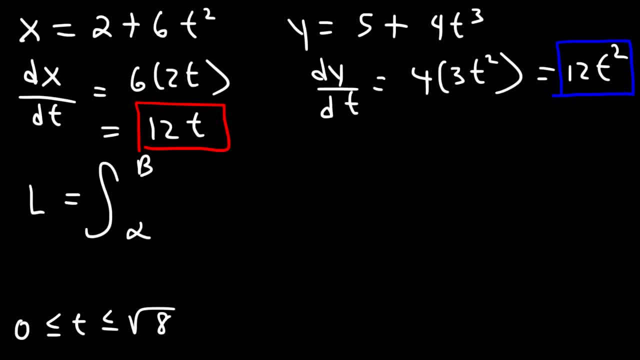 arc length using this formula. So it's the integral from alpha to beta of the square root of dx, dt squared squared, which is 12t, plus dy over dt squared, which is 12t squared squared. Now, alpha is 0 and beta is the square root of 8.. 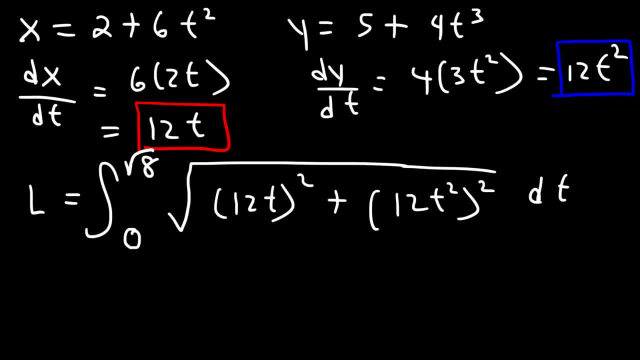 So what can we do to evaluate this integral? Let's begin by simplifying it: 12 squared is 144, so we're going to have 144t squared and 12t squared squared. that's going to be 144 and t squared squared is t. to the fourth power. 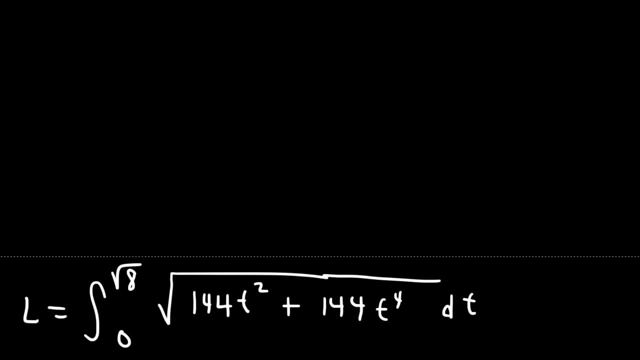 So what do you think we need to do at this point? We need to factor out the greatest common factor inside the square root, and so that's going to be 144t squared. If we take that out, we're going to be left with 1 plus t squared. 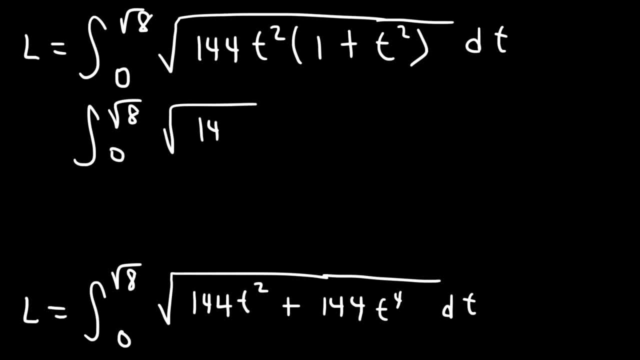 So now, at this point, we can separate this into two radical expressions. The square root of 144 is 12 and the square root of t squared is just t, So we're going to have 12t times this. So how can we integrate this expression? 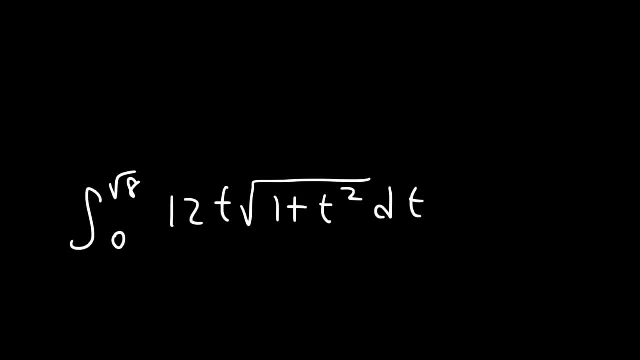 What techniques can we use? I would recommend use substitution. If we set u equal to 1 plus t, squared du is going to be 2t times dt. So solving for dt, that's going to be du over 2t. So we're going to have the integral of 12t times the square root of u. 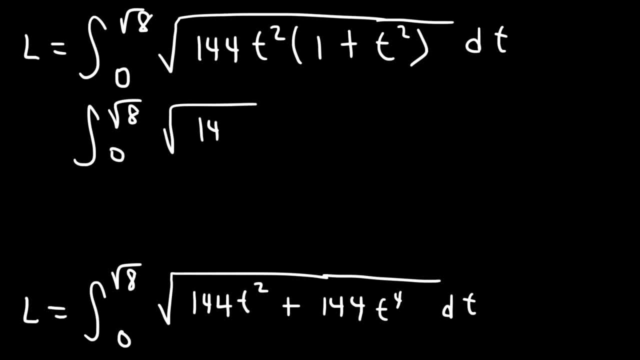 So now, at this point, we can separate this into two radical expressions. The square root of 144 is 12 and the square root of t squared is just t, So we're going to have 12t times this. So how can we integrate this expression? 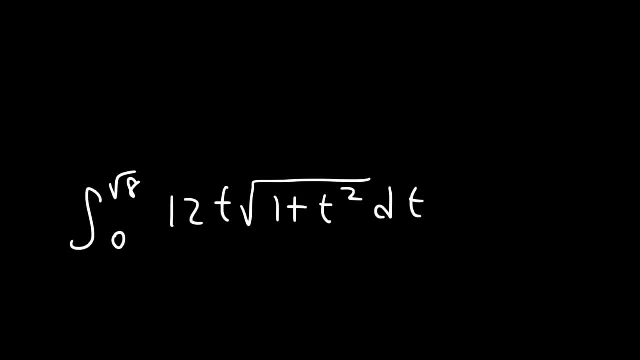 What techniques can we use? I would recommend use substitution. If we set u equal to 1 plus t, squared du is going to be 2t times dt. So solving for dt, that's going to be du over 2t. So we're going to have the integral of 12t times the square root of u. 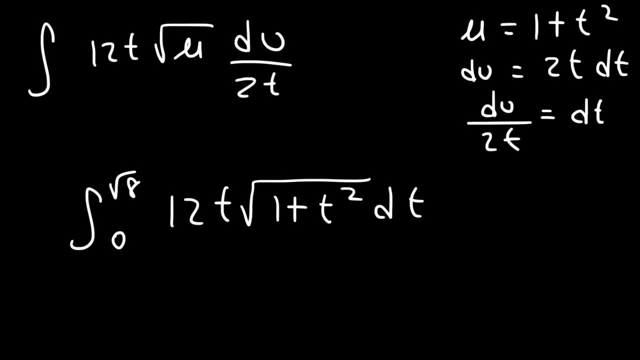 dt squared And we can replace with du over 2t. So we can cancel t And we need to change the limits of integration. So keep in mind: t varied from 0 to the square root of 8.. So let's plug in 0 into this expression. 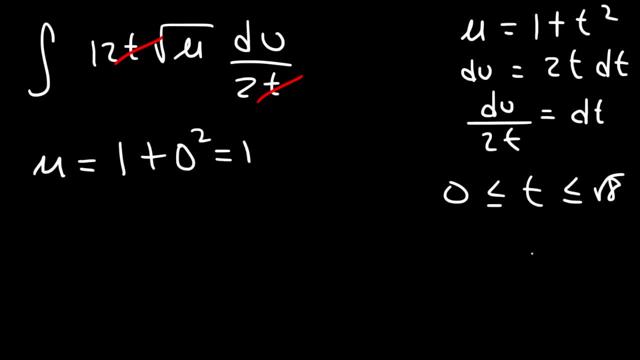 So, replacing t with 0, we're going to have 1 plus 0, squared, which is 1.. And then we're going to have 1 plus 0, squared, which is 1.. And then, replacing t with the square root of 8.. 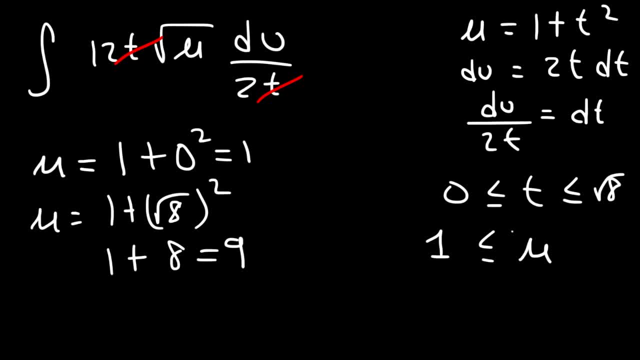 The square root of 8 squared is just 8.. So 1 plus 8 is 9.. So u is between 1 and 9.. Now 12 divided by 2 is 6 and we can move that to the front. 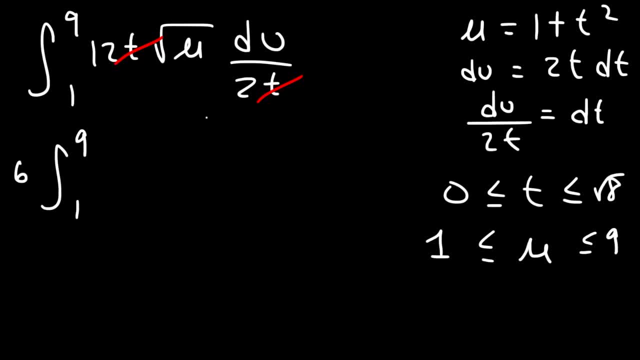 So this is 6 times the integral from 1 to 9.. The square root of u, which is u to the 1 half du. Now let's use the power rule: 1 half plus 1 is 3 over 2.. 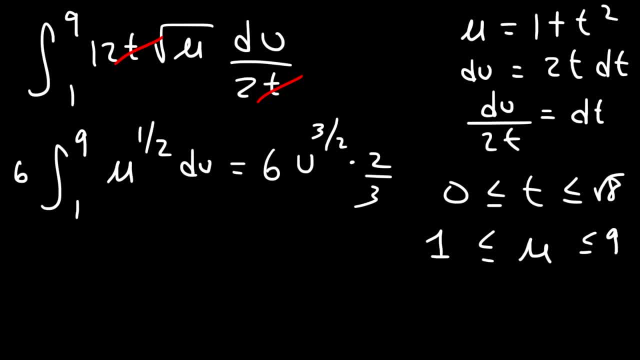 And instead of dividing it by 3 over 2, we're going to multiply it by 2 over 3.. Now 6 divided by 3 is 2.. And then times another 2, that's going to be 4.. So this is equal to 4 times u raised to the 3 over 2, evaluated from 1 to 9.. 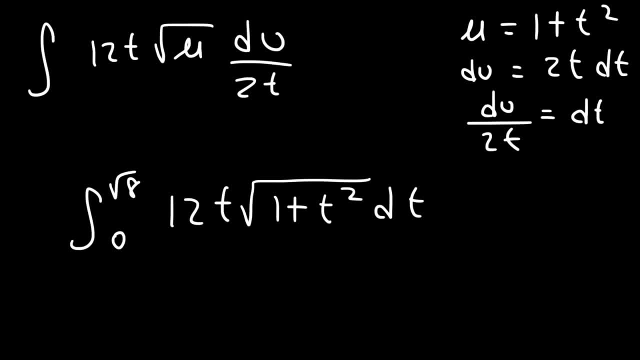 dt squared And that can be replaced with du over 2t, So we can cancel t and we need to change the limits of integration. So keep in mind: t varied from 0 to the square root of 8.. So let's plug in 0 into this expression. 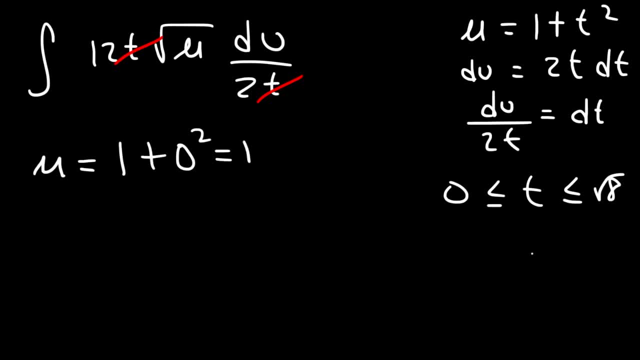 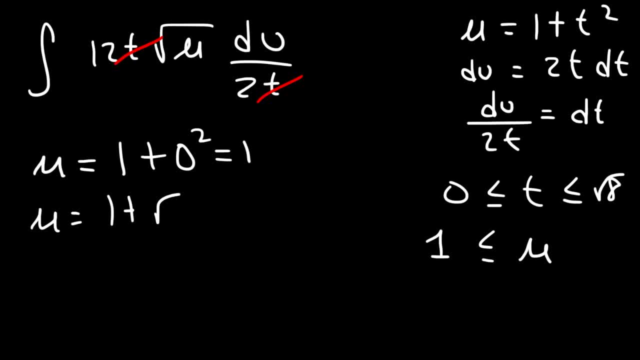 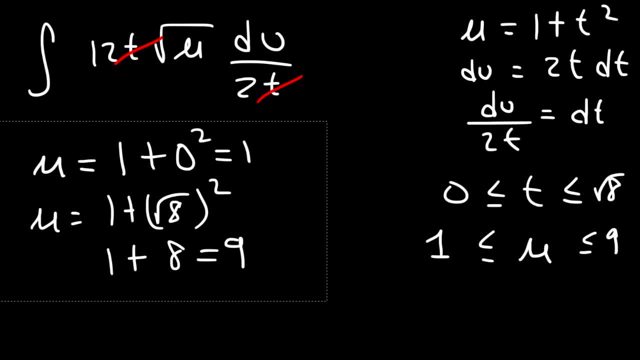 So u is between 1 and 9.. Now 12 divided by 2 is 6 and we can move that to the front. So this is 6 times the integral from 1 to 9, the square root of u, which is u to the one. 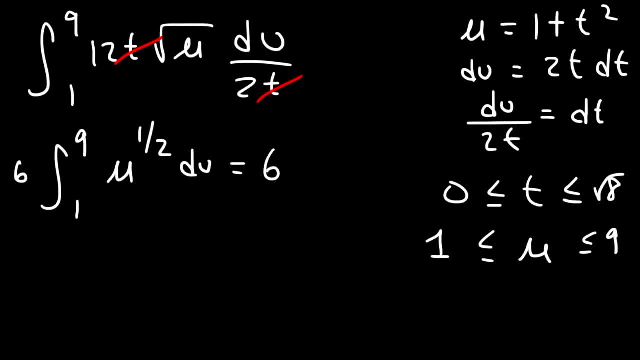 half du. Now let's use the formula: 1 half plus 1 is 3 over 2, and instead of dividing it by 3 over 2, we're going to multiply it by 2 over 3.. Now, 6 divided by 3 is 2, and then times another 2, that's going to be 4.. 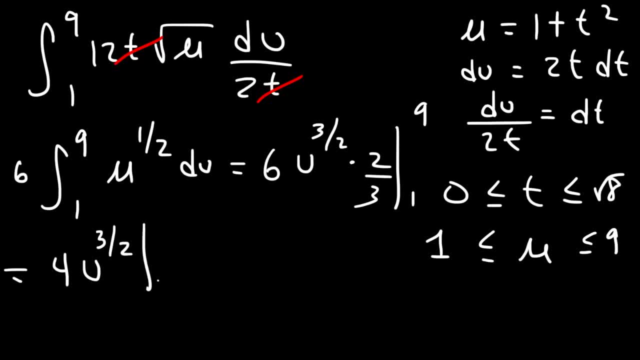 So this is equal to 4 times u raised to the 3 over 2, evaluated from 1 to 9.. So we're going to have 2 times u raised to the 3 over 2, which is 4.. Now let's use the power rule. 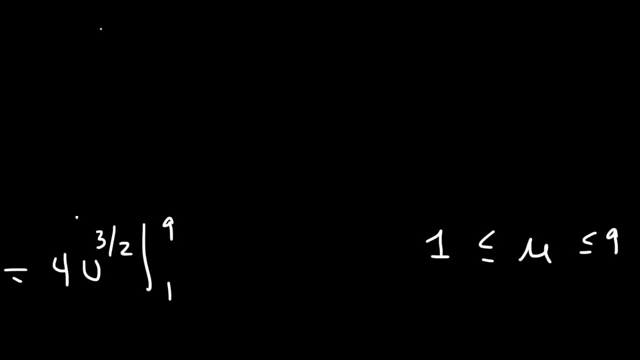 1 half plus 1 is 3 over 2.. And instead of dividing it by 3 over 2, we're going to multiply it by 2 over 3.. So if we plug in 9, it's going to be 9 to the 3 halves and then minus 1 to the 3 halves. 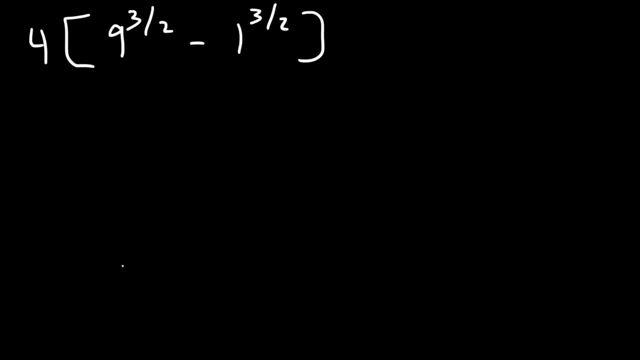 So what is 9 raised to the 3 over 2?? This is the same as 9 raised to the one half. raised to the third power, 9 to the one half is the square root of 9 and the square root of 9 is 3.. 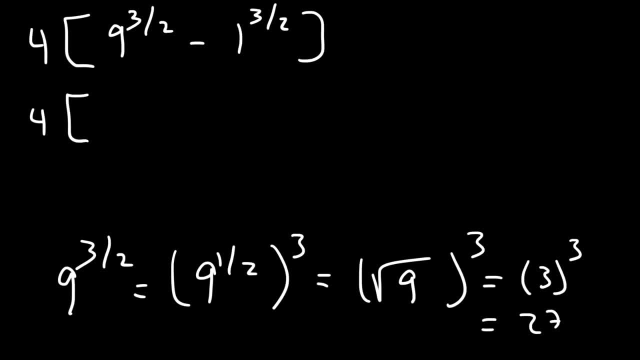 3 to the third power is 27.. So therefore, 9 raised to the 3 over 2 is 9.. So what is 9 raised to the 3 over 2?? 9 raised to the 3 over 2 is 27.. 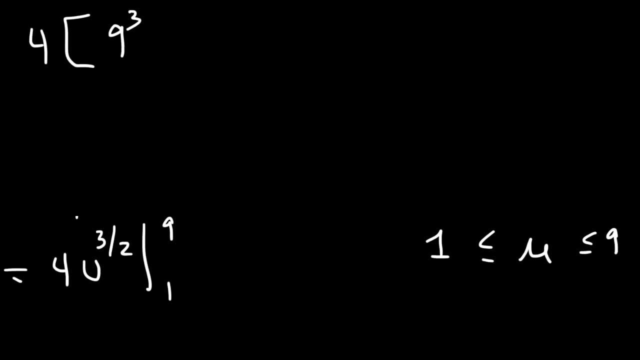 So if we plug in 9, it's going to be 9 to the 3 halves and then minus 1 to the 3 halves. So what is 9 raised to the 3 over 2?? This is the same as 9 raised to the 1 half raised to the 3rd power. 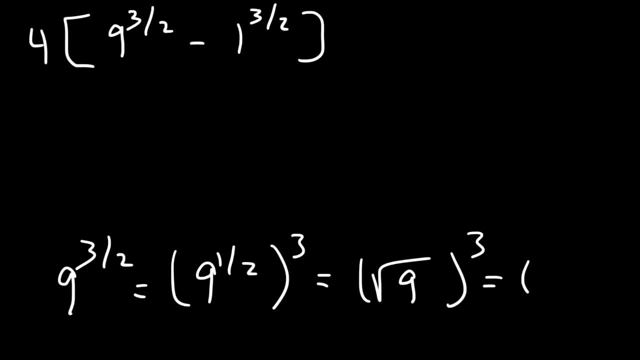 9 to the 1 half is the square root of 9. And the square root of 9 is 3.. 3 to the 3rd power is 27.. So, therefore, 9 raised to the 3 over 2 is 27.. 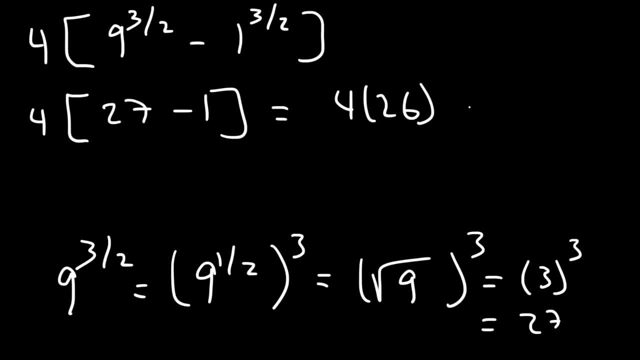 7 minus 1 is 26.. And 26 times 4 is 104.. And that is the answer. That is the length of the arc, as t increases from 0 to the square root of 8.. So now let's work on another example. 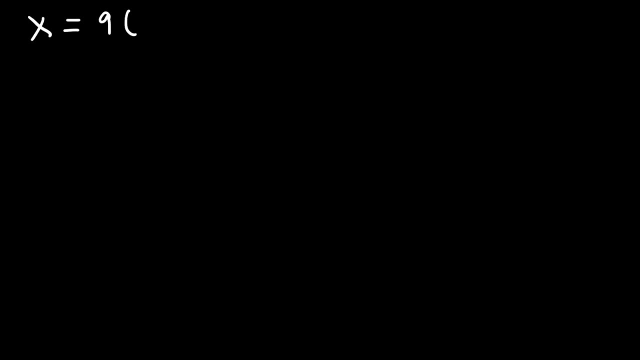 So let's say that x is equal to 9t squared and y is equal to 9t minus 3t to the 3rd power. And let's say we want to find the length of the arc from 0 to 2.. 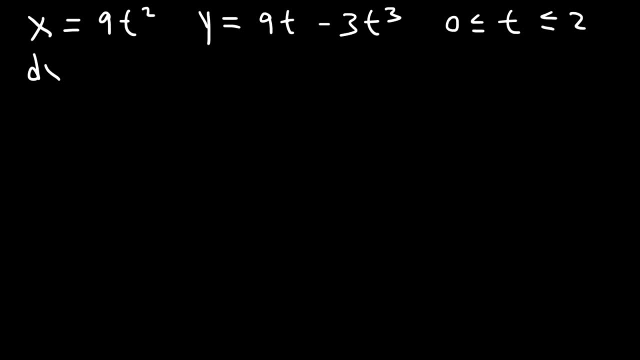 So go ahead and try this problem Now. the first thing I'm going to do is calculate or determine dx dt. dx dt is going to be 18t, and then I'm going to find dy dt, which is 9 minus 9t squared. 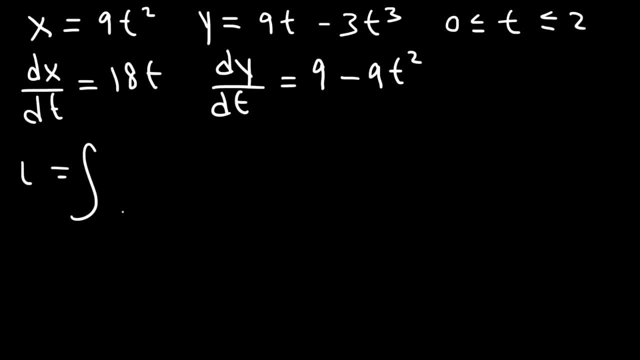 So now let's go ahead and use the formula. So the arc length is going to be from alpha to beta. So the length of the arc length is going to be from alpha to beta. So the length of the arc length is going to be from alpha to beta. 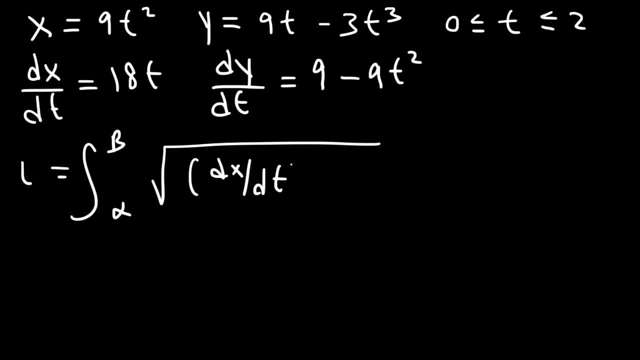 And we're going to have the square root of dx dt squared plus dy dt squared. So, using that formula, we're going to have the integral from 0 to 2 square root, 18t squared plus. Now for dy dt. simplify: we can take out a nine and so we'll have one minus T squared. it's 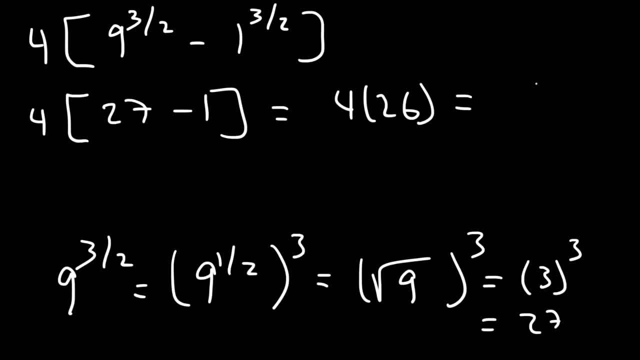 And 27 minus 1 is 26.. And 26 times 4 is 104.. And that is the answer. That is the length of the arc, as t increases from 0 to the square root of 8.. So now let's work on another example. 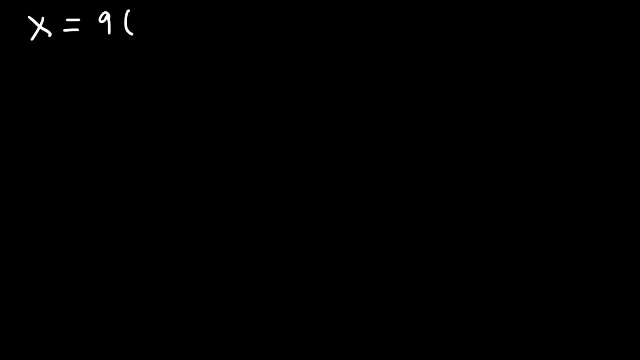 So let's say that x is equal to 9t squared and y is equal to 9t minus 3t squared. So we're going to have 9 raised to the 3 over 2.. And instead of dividing it by 3 over 2, we're going to multiply it by 9 to the 3 halves. 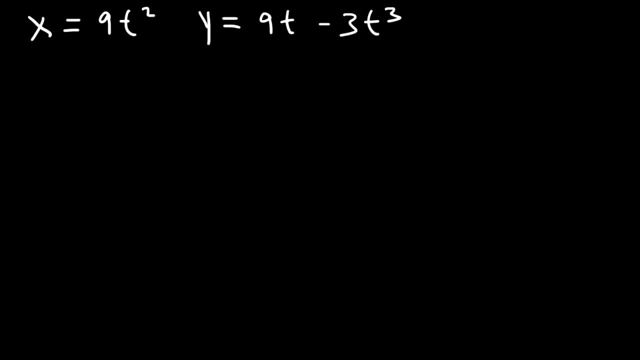 So what is 9 raised to the 3 over 2?? 9 raised to the 3 over 2 is 9t to the third power. And let's say we want to find the length of the arc from 0 to 2.. 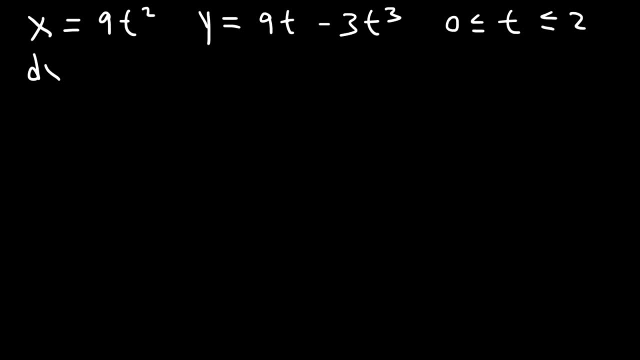 So go ahead and try this problem Now. the first thing I'm going to do is calculate or determine dx dt. Dx dt is going to be 18t, and then I'm going to find dy dt, which is 9 minus 9t squared. 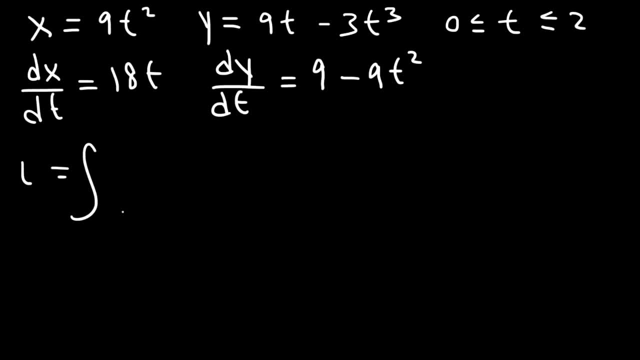 So now let's go ahead and use the formula. 9 is going to be, from alpha to beta, the square root of dx- dt squared plus dy- dt squared. So using that formula, we're going to have the integral from 0 to 2 square root, 18t squared. 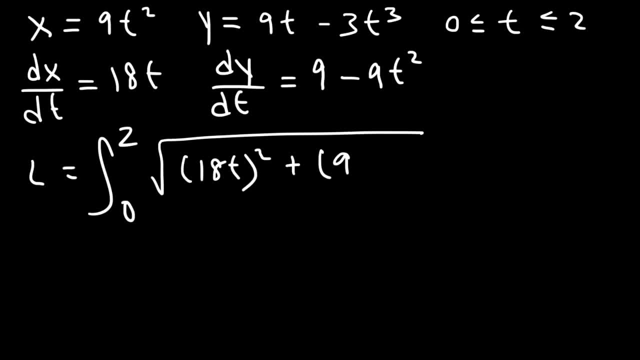 plus 18t squared. Now for dy dt. let's simplify it. We can take out a 9, and so we'll have 1 minus t squared. It's better if we put it in that form, because it's going to be easy to find the square of. 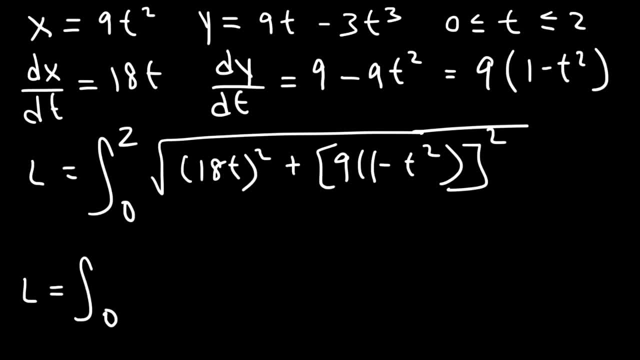 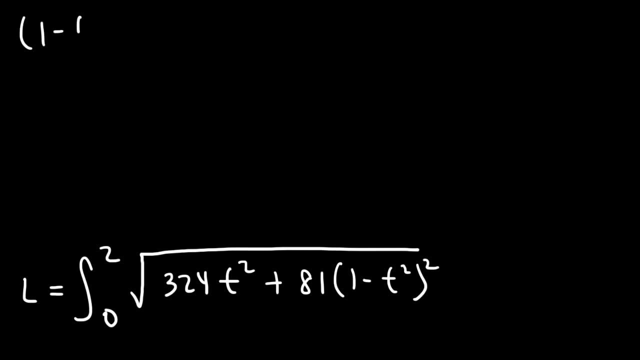 that expression, 18 squared is 324.. 9 squared is 81.. And so we're going to have 81 squared, And so we're going to have 81 squared, And so we're going to have 81 times 1 minus t squared squared. 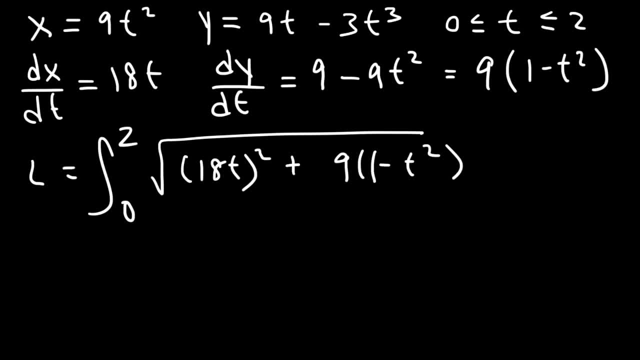 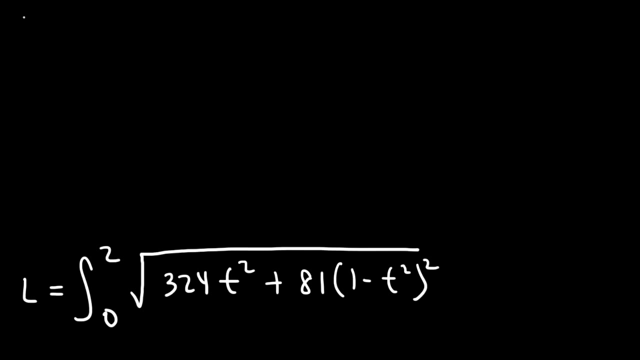 better if we put it in that form, because it's going to be easy to find a square of that expression: 18 squared is 324, 9 squared is 81, and so we're going to have 81 times 1 minus T squared squared. one minus T squared squared is basically 1 minus T squared times 1 minus T. 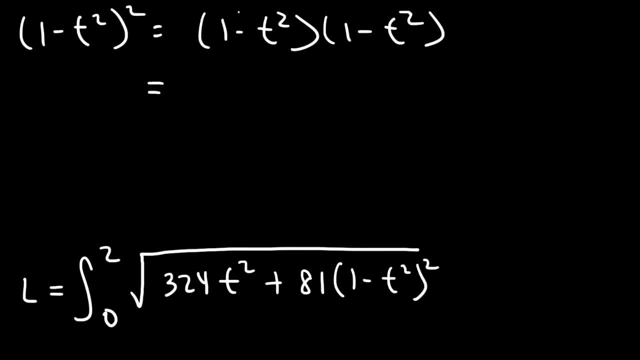 squared. so if we foil this expression, 1 times 1 is 1, and then we'll have 1 times negative T squared, and then this will give us negative T squared and then plus T to the fourth. so that's 1 minus 2 T squared, plus T to the fourth. 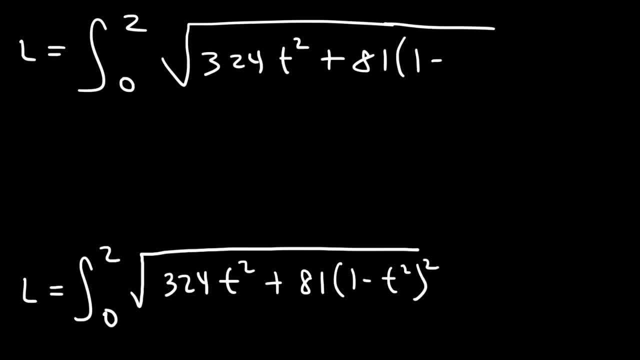 so we're gonna have 81 times 1 minus 2 T squared plus T to the fourth. so what we need to do at this point is distribute the 81, so it's gonna be 81 minus 162 T, squared plus 81 T to the fourth. 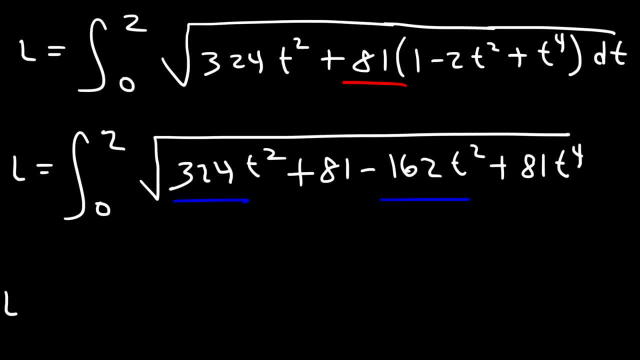 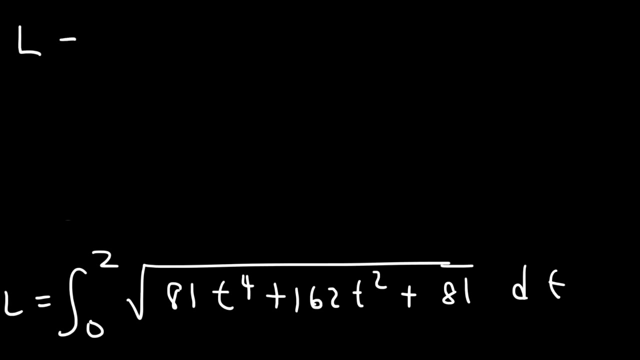 now let's combine like terms and put this in standard form. So this is 81T to the 4th, 324 minus 162, that's positive 162. Now we need to take out an 81. So if we factor out the GCF, we're going to have T to the 4th and then 162 divided by 81, that's 2.. 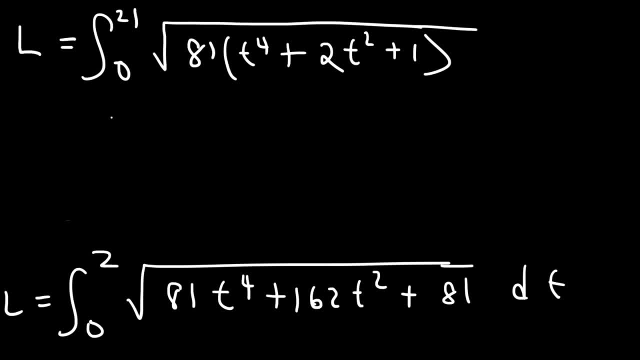 So plus 2T squared, and then plus 1.. Now, at this point, because the 81 is multiplied by T to the 4th, plus 2T squared plus 1, we can separate it into two radicals. Now, what do you think we need to do at this point? What is our next step? 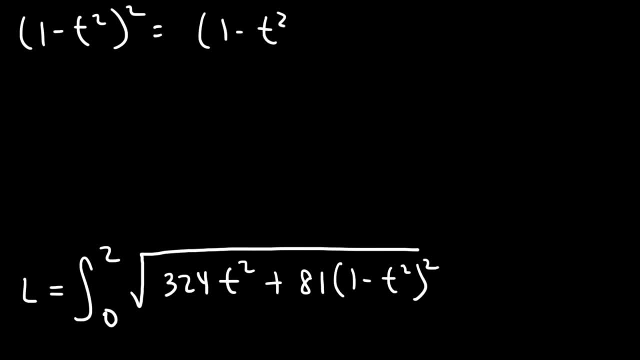 1 minus t squared squared is basically 1 minus t squared times 1 minus t squared. So if we FOIL this expression, 1 times 1 is 1, and then we'll have 1 times negative t squared and then this will give us negative t squared and then plus t to the fourth. 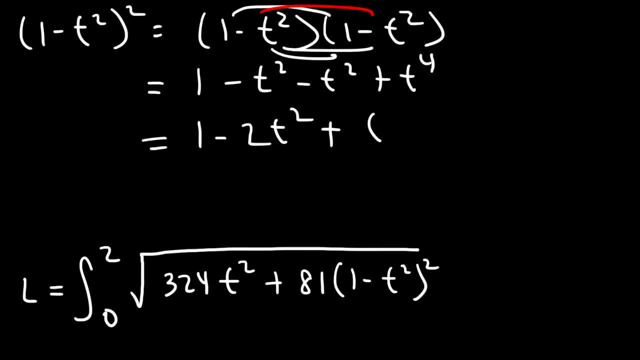 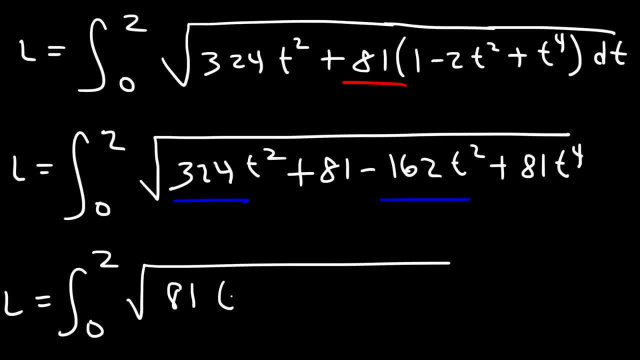 And so we're going to have 81 times 1 minus 2 t squared plus t to the fourth. And so we're going to have 81 times 1 minus 2 t squared plus t to the fourth. So this is 81t to the 4th, 324 minus 162, that's positive 162.. 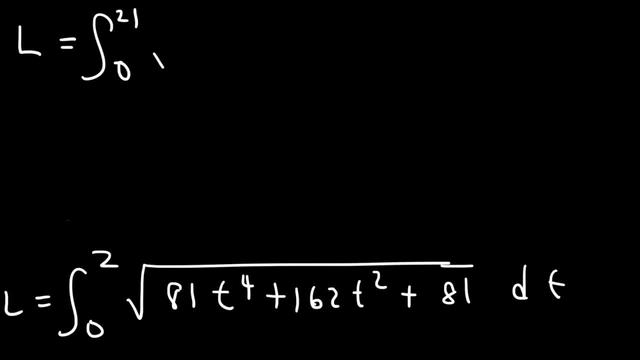 Now we need to take out an 81. So if we factor out the GCF, we're going to have t to the 4th and then 162 divided by 81, that's 2.. So plus 2t squared, and then plus 1.. 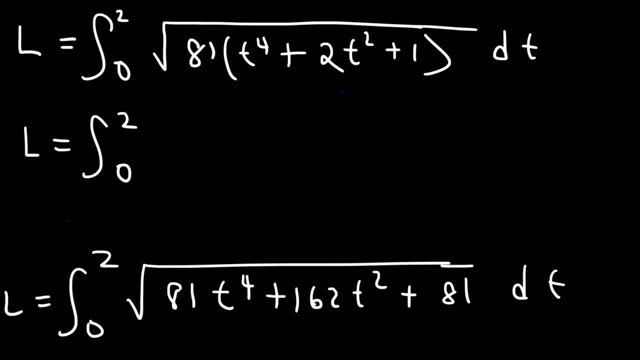 Now at this point, because the 81 is multiplied by t to the 4th plus 2t squared plus 1, we can separate it into two radicals. Now, what do you think we need to do at this point? What is our next step? 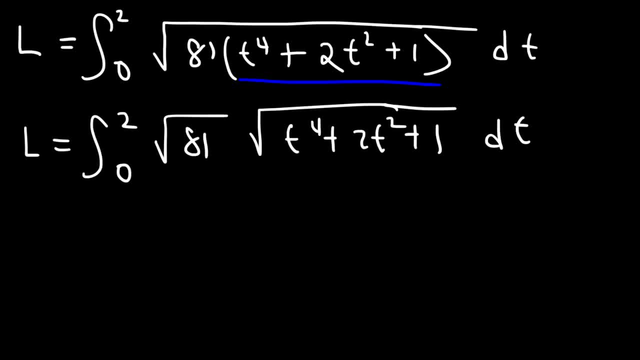 Notice that we can. We can factor t to the 4th plus 2t squared plus 1.. The square root of 81 is 9. And we can factor it this way: It's t squared plus 1 times t squared plus 1.. 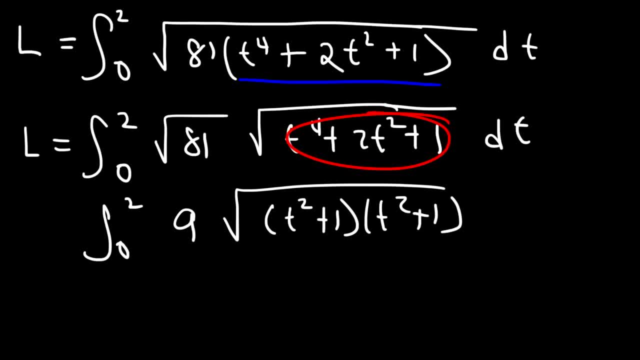 If you FOIL it, you're going to get this expression. It's a perfect square trinomial, so to speak, So we can write it as t squared plus 1 squared, And so the square root of t, squared plus 1 squared. 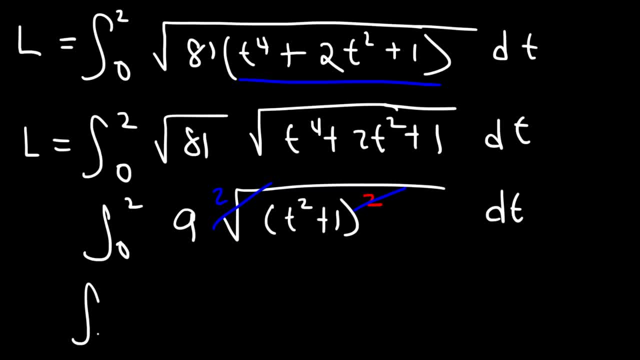 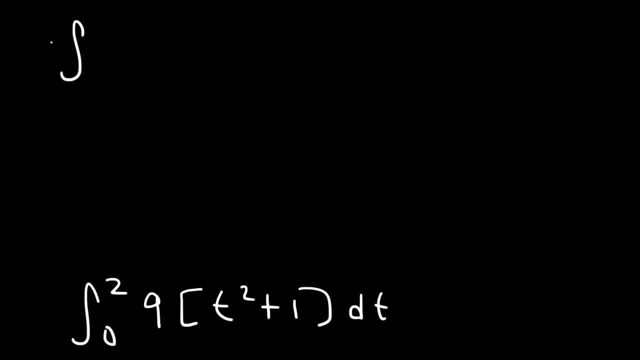 the square root and the square will cancel, And so we're going to have the integral from 0 to 2, 9 times t squared plus 1 dt. So let's go ahead and distribute the 9.. Actually, let's move the 9 to the front. 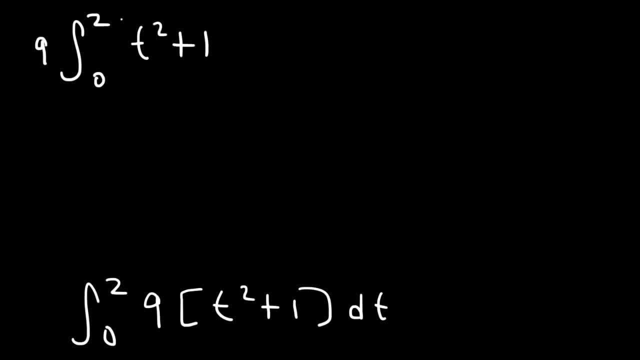 That's going to be a lot easier, And so this is what we now have. Now we can find the antiderivative of t squared, So that's t to the 3rd divided by 3.. And the antiderivative of 1 is t. 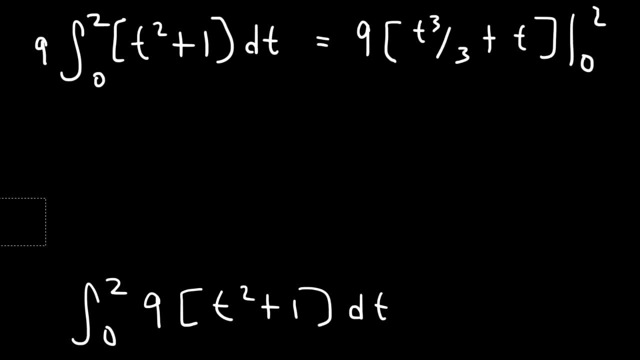 So we evaluate it from 0 to 2.. So let's plug in 2.. So it's going to be 2 to the 3rd, which is 8, divided by 3, plus 2.. And then we need to plug in 0.. 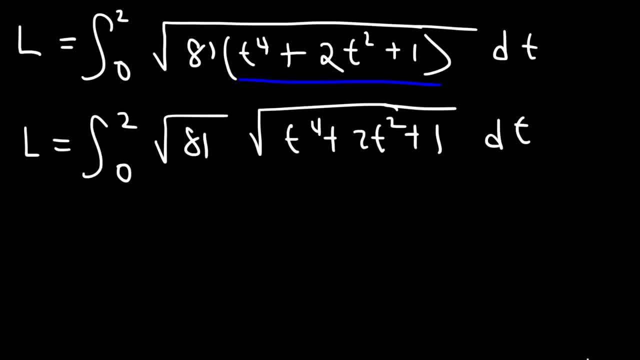 Notice that we can separate the 81 to the 4th. We can factor T to the 4th plus 2T squared plus 1.. The square root of 81 is 9. And we can factor it this way: It's T squared plus 1 times T squared plus 1.. 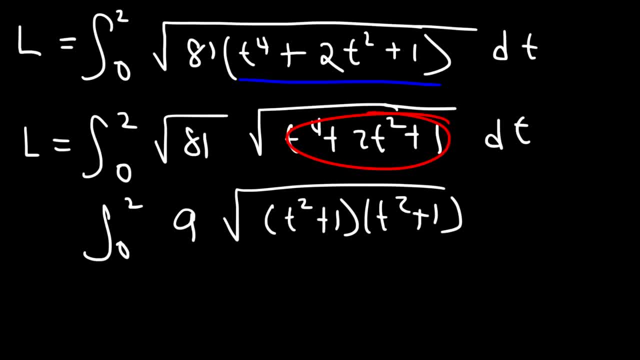 If you FOIL it, you're going to get this expression. It's a perfect square trinomial, so to speak, So we can write it as T squared plus 1 squared, And so the square root of T squared plus 1 squared. the square root and the square will cancel. 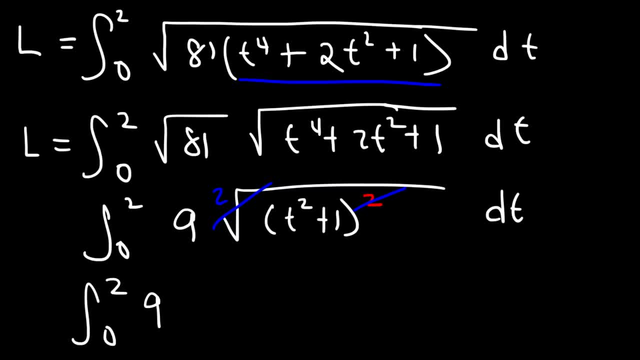 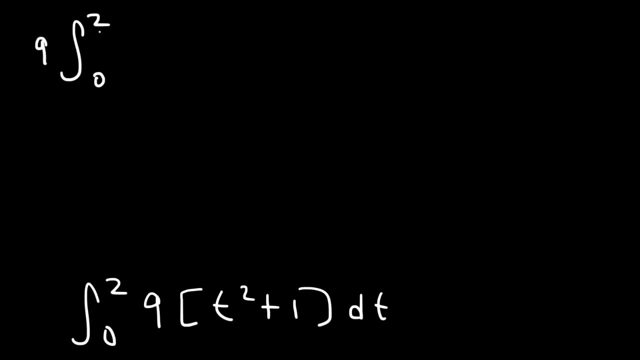 And so we're going to have the integral from 0 to 2, 9 times T squared plus 1, DT. So let's go ahead and distribute the 9.. Actually, let's move the 9 to the front. That's going to be a lot easier. 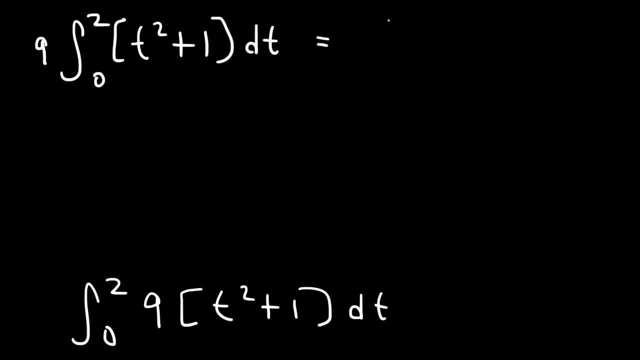 And so this is what we now have. Now we can find the antiderivative of T squared, so that's T to the 3rd divided by 3.. And the antiderivative of 1 is T. So we evaluate it from 0 to 2.. 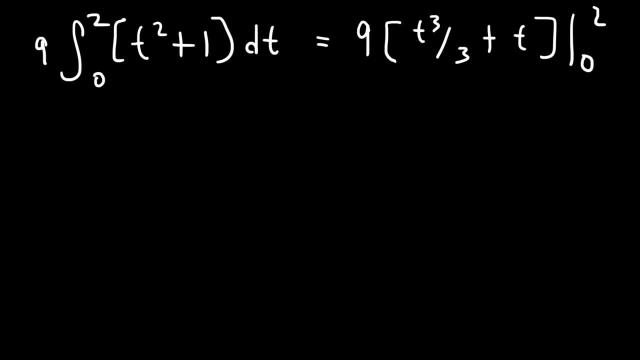 So let's plug in 2.. So it's going to be 2 to the 3rd, which is 8, divided by 3, plus 2.. And then we need to plug in 0. So 0 to the 3rd is just 0 plus T, which is 0.. 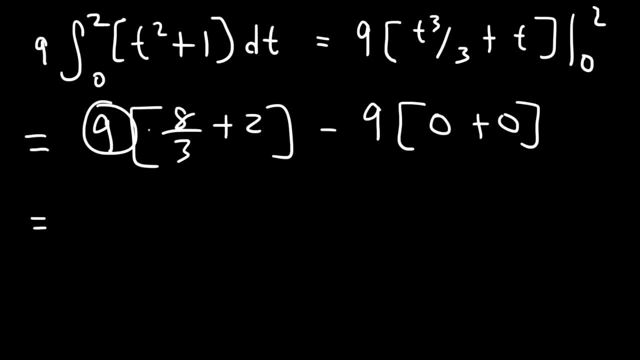 So that whole thing is 0.. 9 divided by 3 is 3. And 3 times 8 is 24.. And then 9 times 2 is 18.. And then 24 plus 18,, that's 42.. 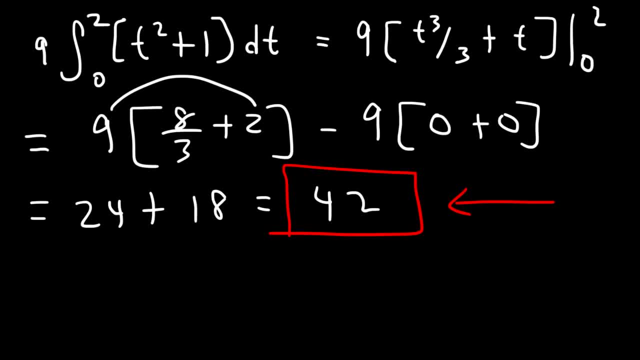 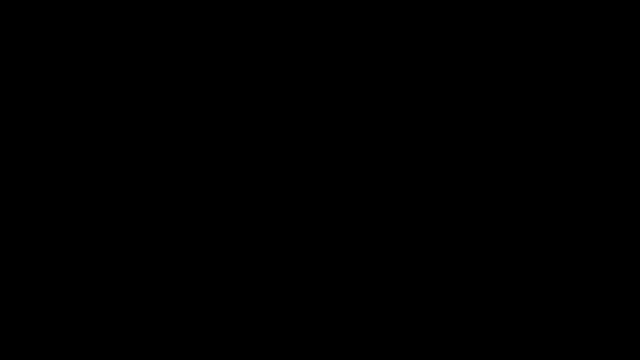 So this is the length of the arc And so that's it for this video And I hope you enjoyed it And I hope you found it useful, And I hope you found it helpful. And I hope you found it helpful. And I hope you found it useful. 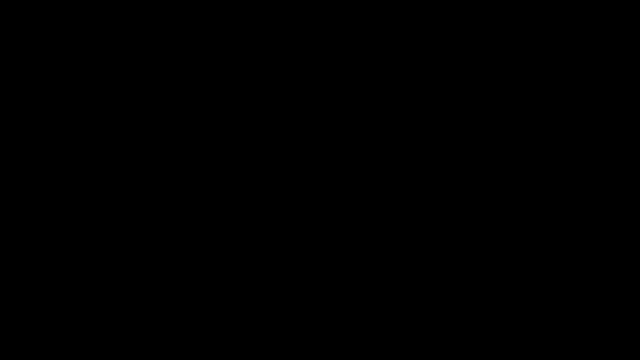 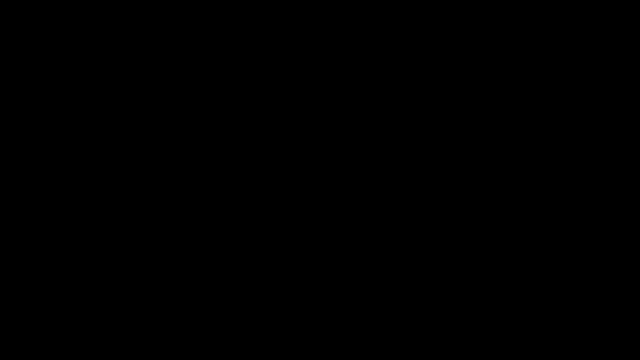